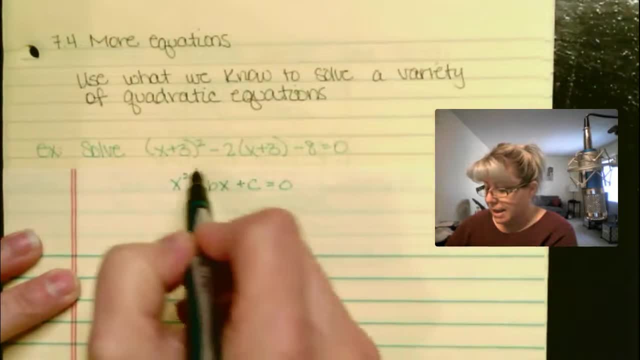 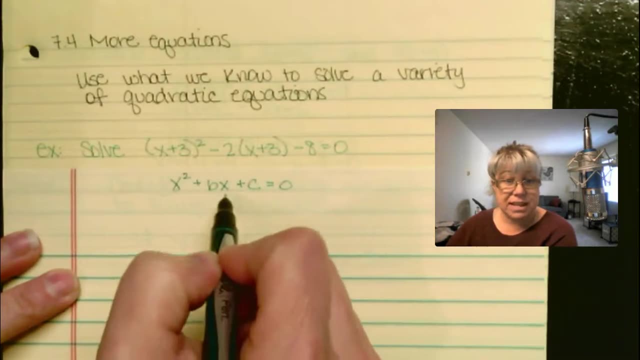 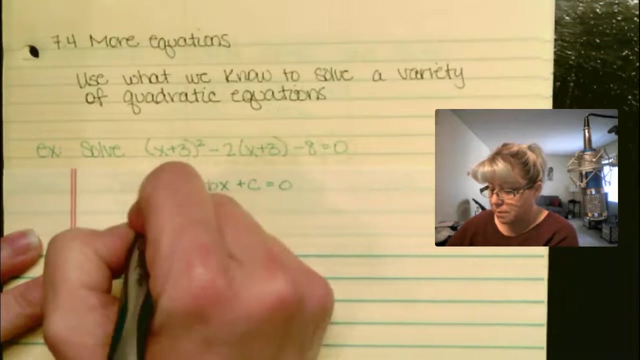 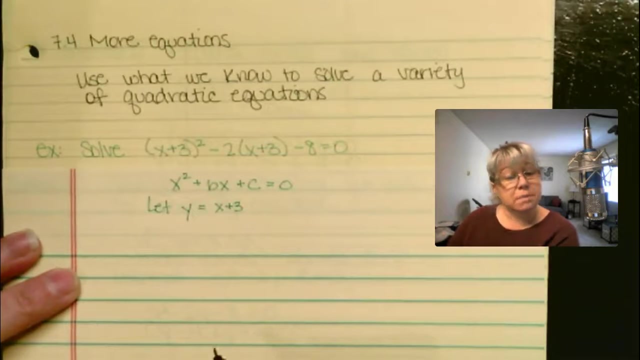 equals 0,, this kind of x-looking thing looks like x plus 3.. This x looks like x plus 3.. So why not? let's simplify this problem by Let y equal x plus 3.. And we'll substitute in: wherever we see an x plus 3, we'll substitute in y. 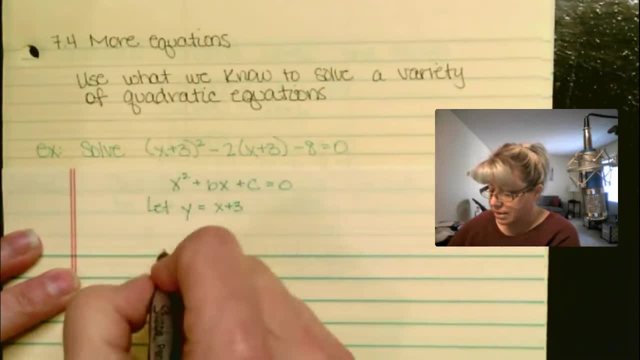 Alright, x plus 3 squared, that's going to become y squared minus 2x plus 3.. Well, x plus 3 is y, so let's substitute in: y Minus 8 equals 0.. Now, certainly, y squared minus 2y minus 8 is. 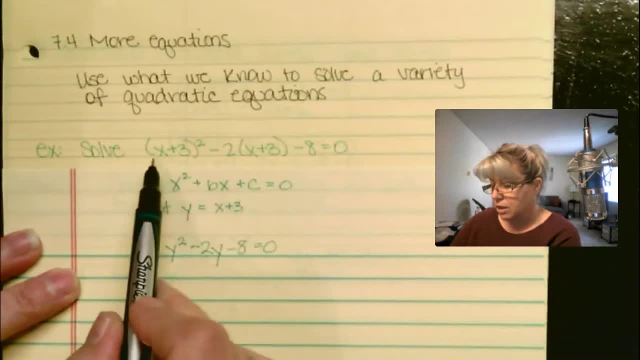 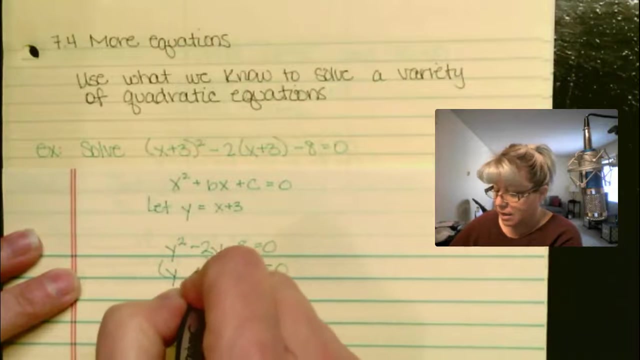 a lot simpler looking than x plus 3 squared minus 2 times x plus 3 minus 8.. So let's go ahead and factor and solve our simpler or less complex quadratic equation. y and y will get us x squared, two numbers that multiply to negative 8, but add to a negative 2.. 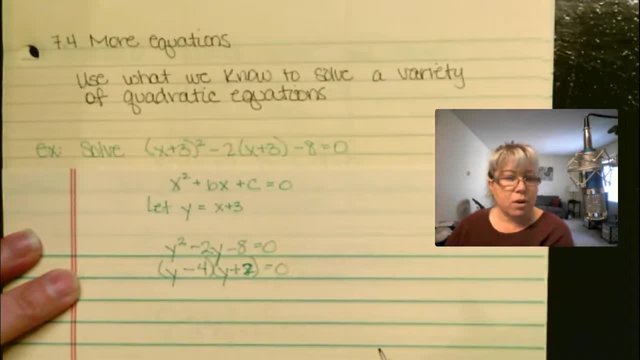 So y minus 4 and y plus 2.. Now let's solve: y minus 4 equals 0 and y plus 2 equals 0.. That means our solutions are: y equals 4 and y equals negative 2.. But I didn't start off with y, I started off with x's and in fact I started off with x plus 3's. So wherever I see a y now, 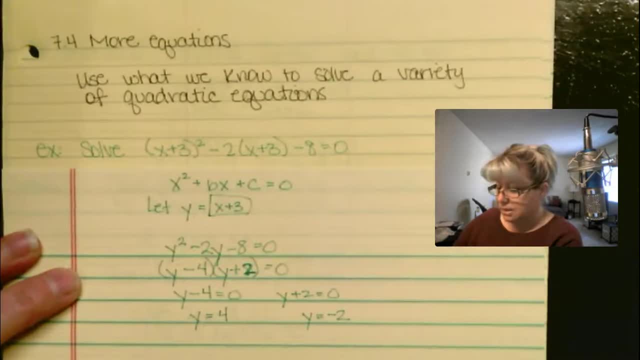 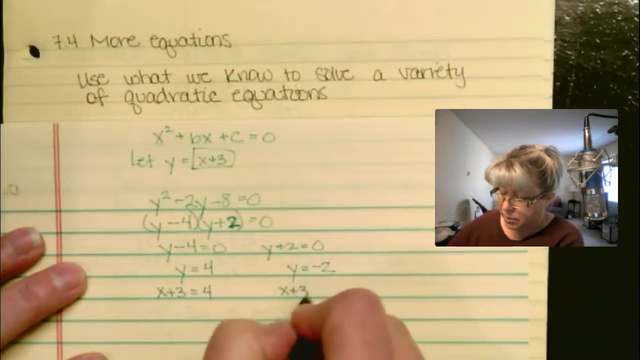 I'm going to substitute back in x plus 3.. x plus 3 equals 4 and x plus 3 equals negative 2.. Now let's solve for x Minus 3 minus 3, x equals 1.. Minus 3 minus 3- over here, x equals negative 5.. 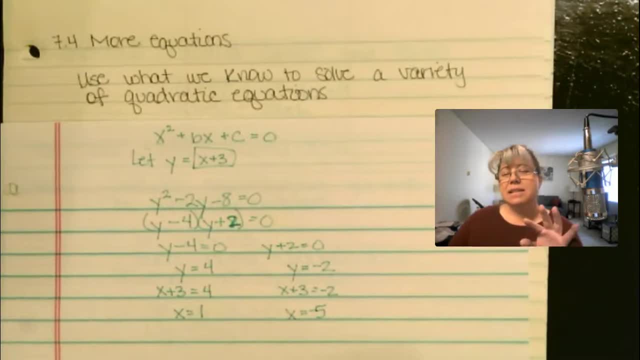 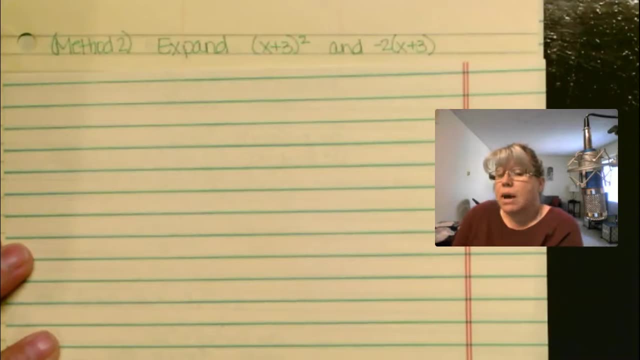 So we can find the solution by simplifying our problem a little by substituting in another variable. That was one way of solving for the solutions. The other is: let's go ahead and expand both x plus 3 and the negative 2 times x plus 3 and combine like terms. 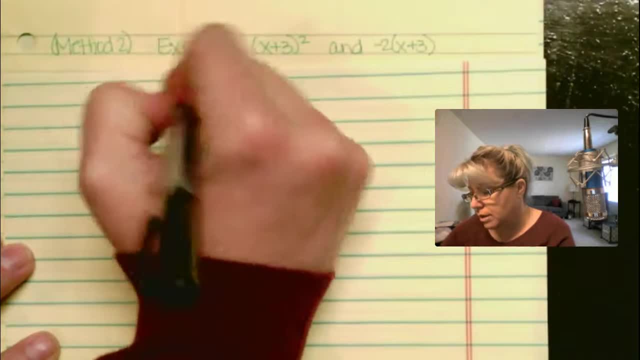 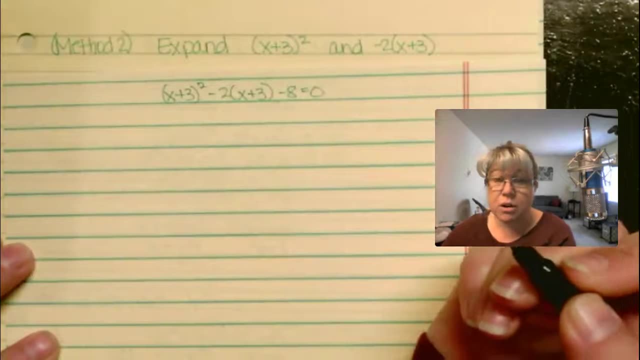 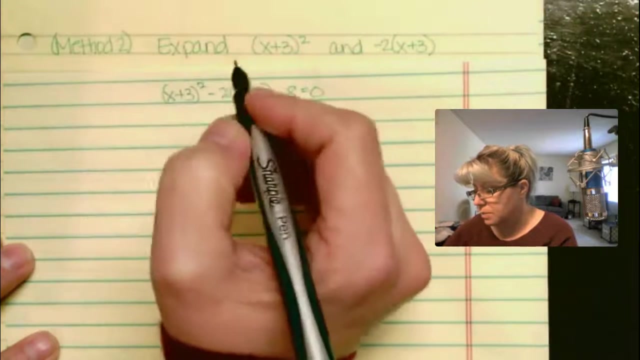 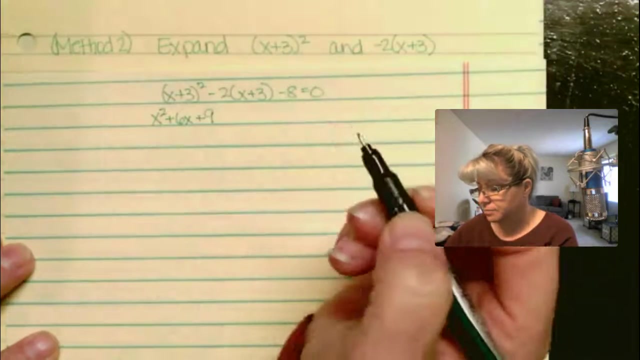 So we had x plus 3, quantity squared minus 2. times x plus 3 minus 8 equals 0, is our answer? original quadratic equation. so I'm going to go ahead and expand the x plus 3 squared. that's going to be x squared plus 6x plus 9. I'm going to go ahead and. 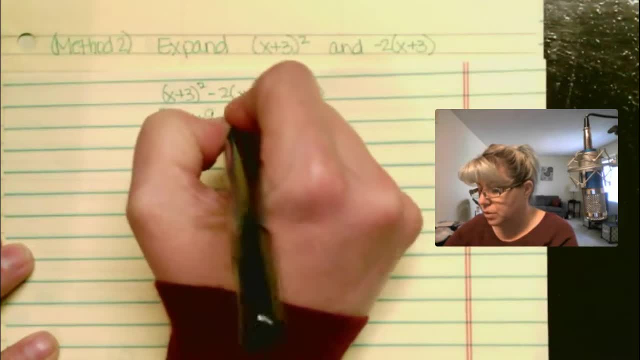 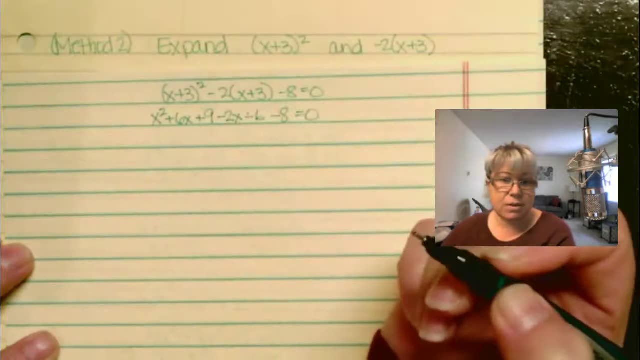 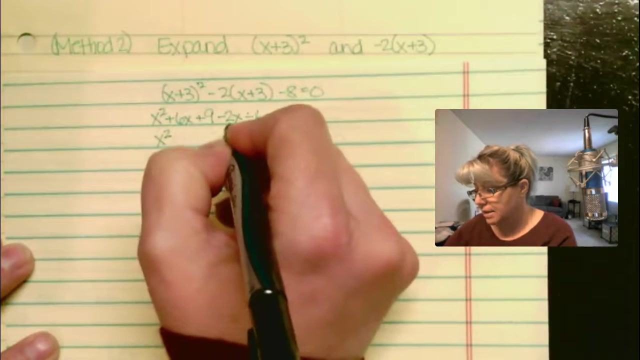 distribute the negative 2 throughout, so negative 2x. negative 2 times 3 is negative. 6 minus 8 equals 0. I need to simplify the left-hand side: x squared, I have a 6x and a minus 2x, which is a positive 4x. I have a plus 9 minus 6. 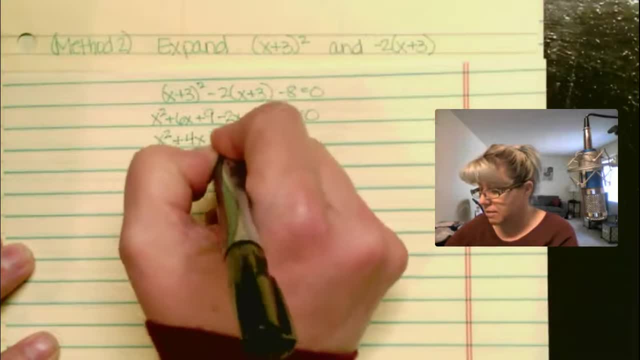 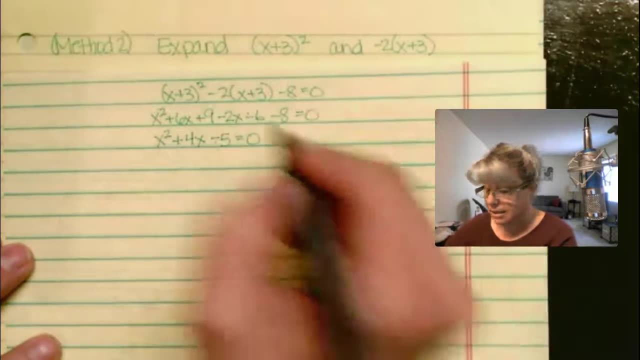 which is 3 minus 8, is minus 5, equals 0. and now that I have the left-hand side as simplified as I can get, I'm going to go ahead and distribute: the x squared plus 3 squared plus 9 minus 8 is minus 5 equals 0. and now that I have the left hand side as simplified as I can get, I'm going to go ahead and. 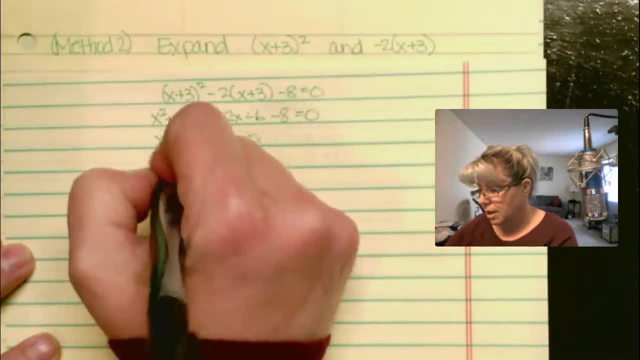 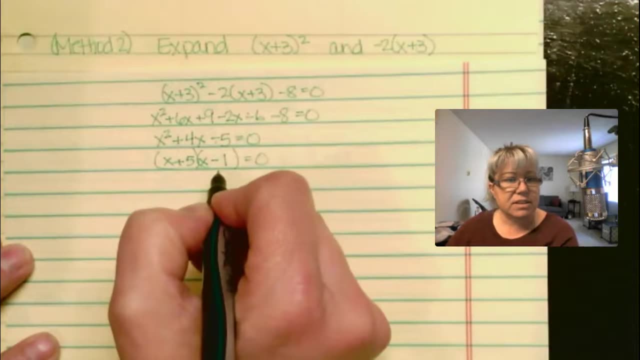 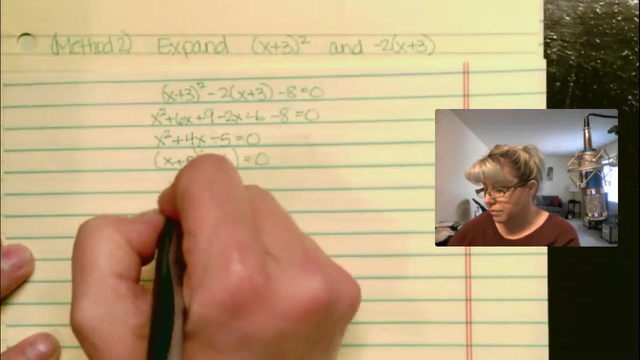 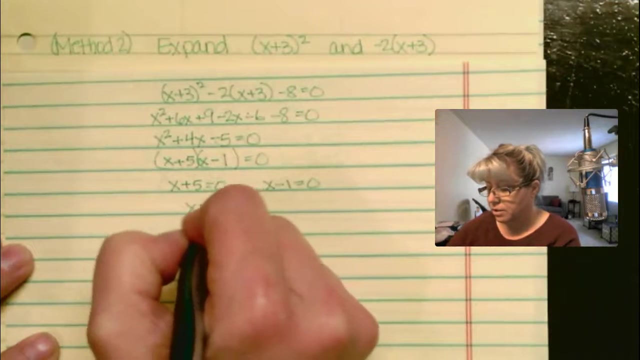 factor: xx plus 5 minus 1, positive 5 times negative. 1 is negative 5, but positive 5 minus 1 is positive 4. and let's solve: x plus 5 equals 0 and x minus 1 equals 0. therefore, our solutions are: x equals negative 5 and x equals 1, same. 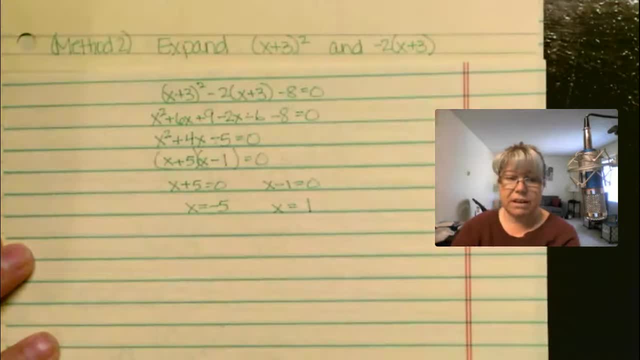 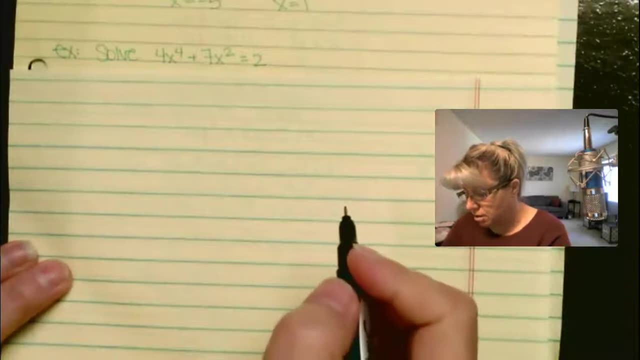 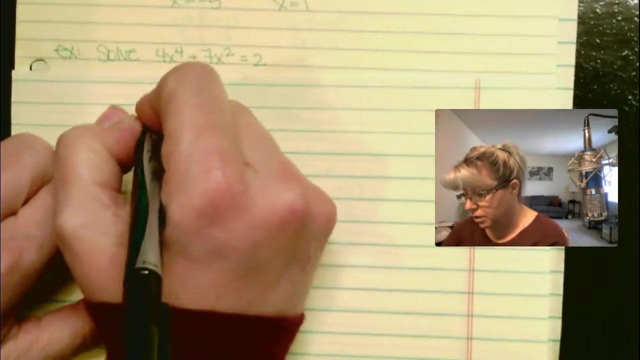 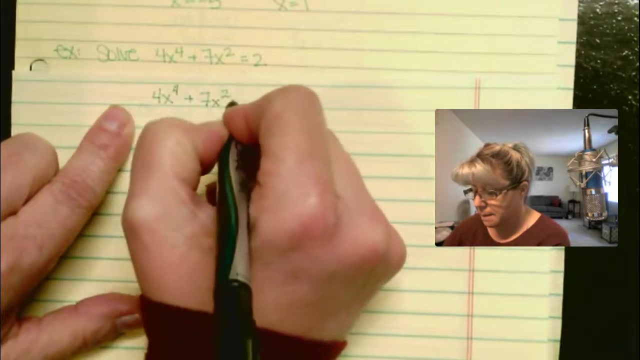 solutions, just two different methods of solving. okay. so let's look at another quadratic equation and solve first off. always has to be in standard form, or at least for the method that I'm thinking about solving using to solve 4x to the fourth, plus 7x squared minus 2 equals 0. now 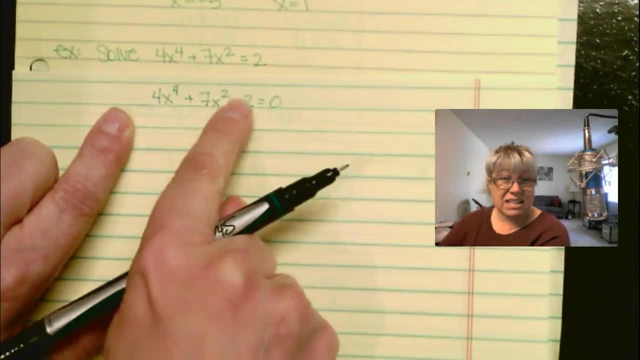 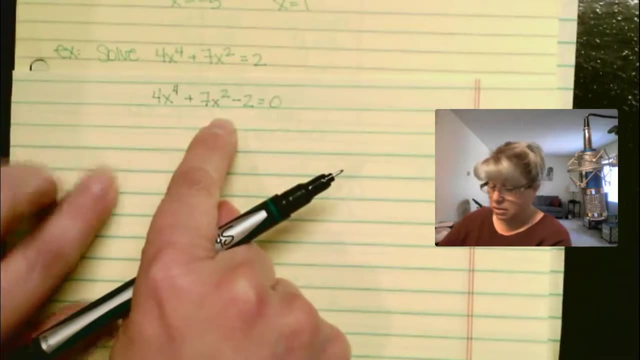 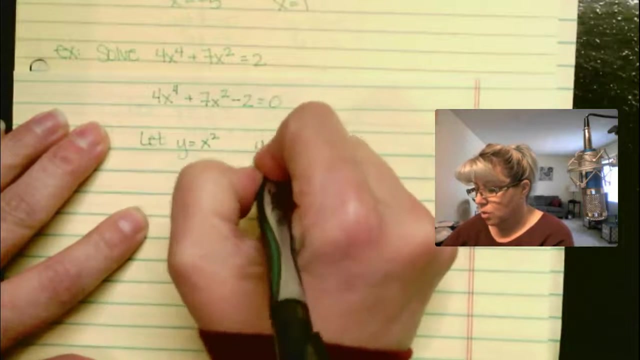 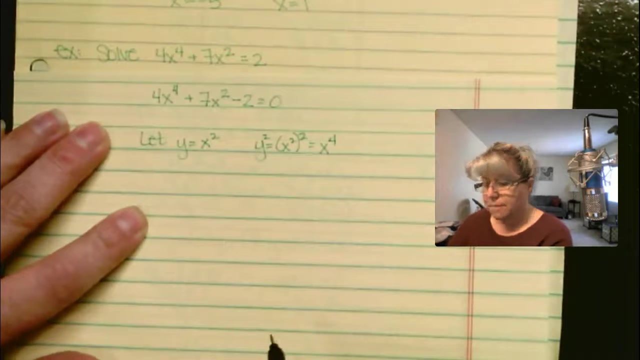 there are x to the fourth and x squared. that is not an x squared and an x, but I can use substitution. if I let y equal x squared, then y squared will equal x squared squared, which is x to the fourth, and I can rewrite this problem using my y. 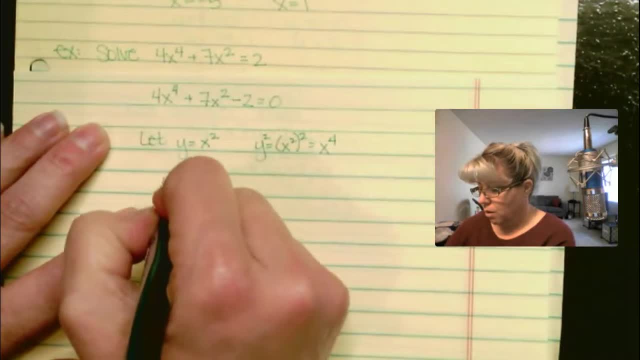 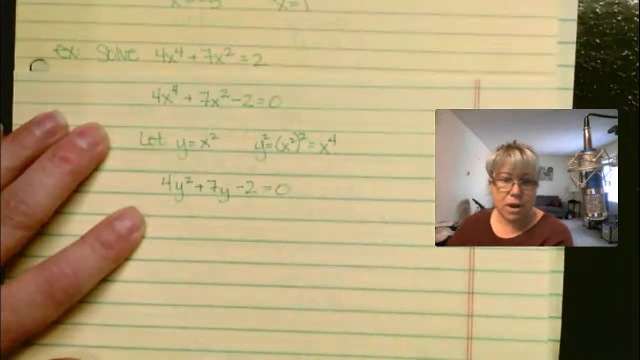 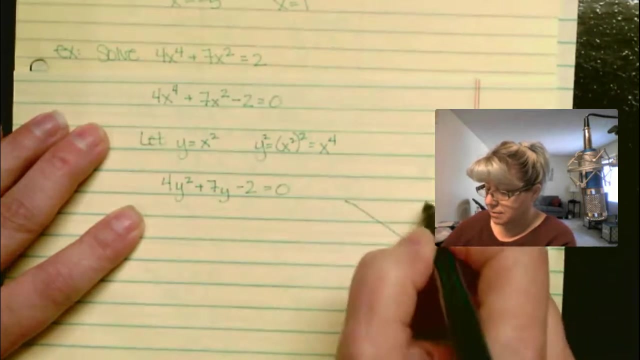 and my y squared, 4y squared plus 7y minus 2 equals 0. now I'm going to use: let's see, let's factor this 4 times negative 2 is negative 8 with a 7. so I'm looking for two numbers. 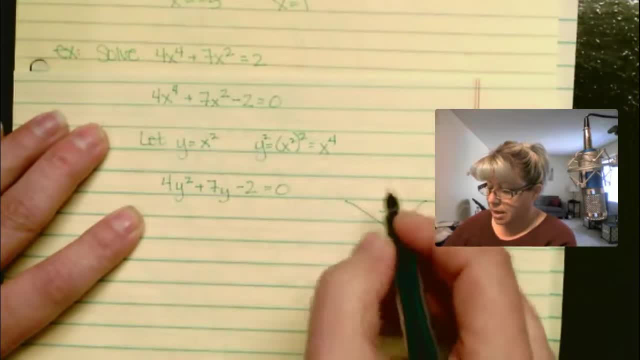 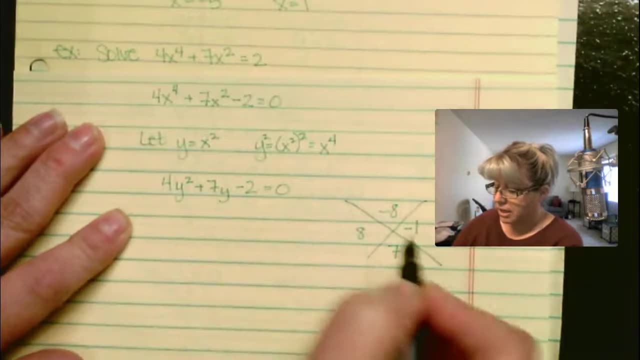 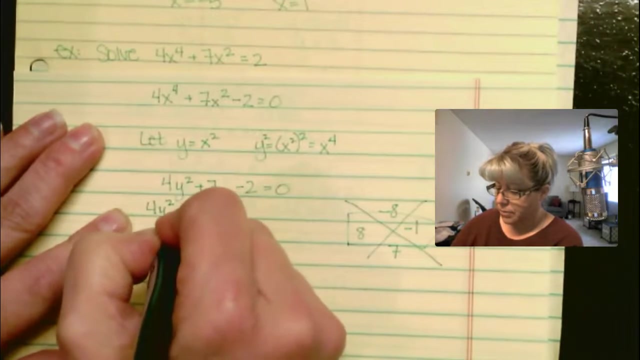 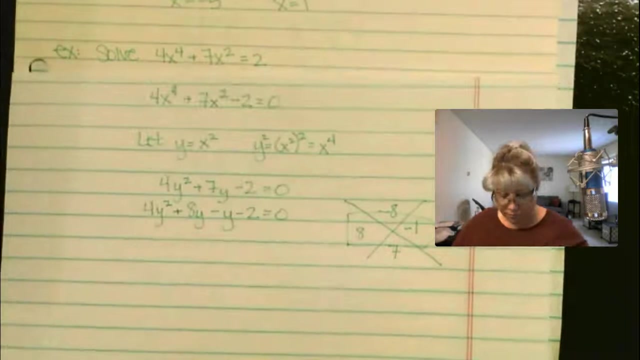 that multiply to negative 8 but add to 7. I think 8 and negative 1 would do the trick. so let's write the middle term in terms of the 8 and negative 1. so 4y squared plus 8y minus y, minus 2, equals 0. now I'm going to take the first two terms and 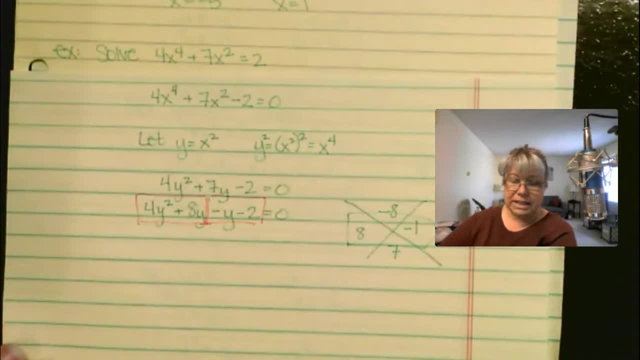 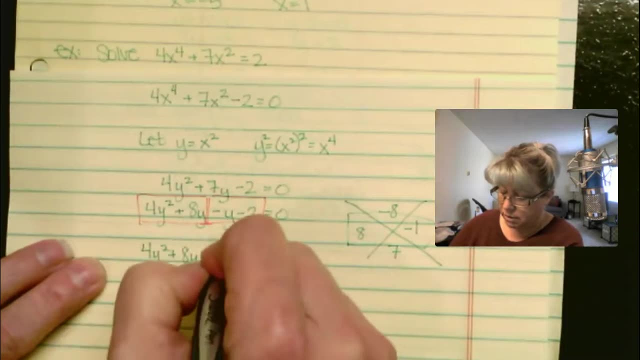 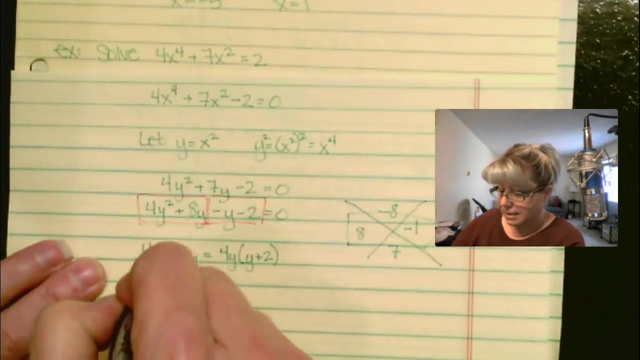 the second two terms and factor each of those terms set of terms. 4y squared plus 8y will equal 4y times y plus 2 and negative y minus 2 will factor into. I can pull out a negative 1, factor out a negative 1, y plus 2. each has a y plus 2 in common, so let's factor y plus 2 for y. 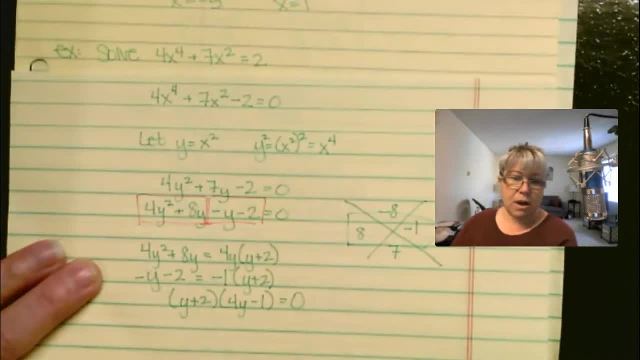 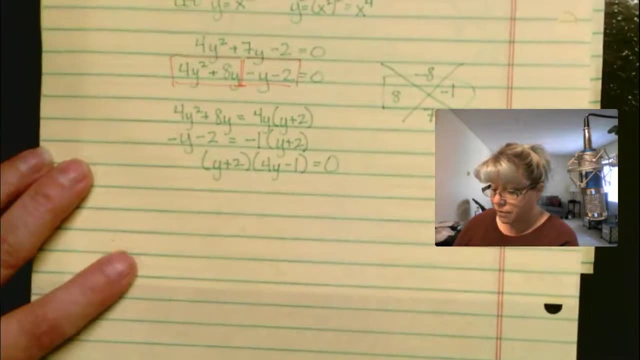 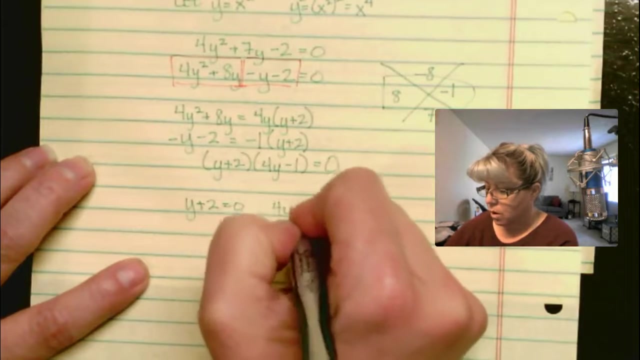 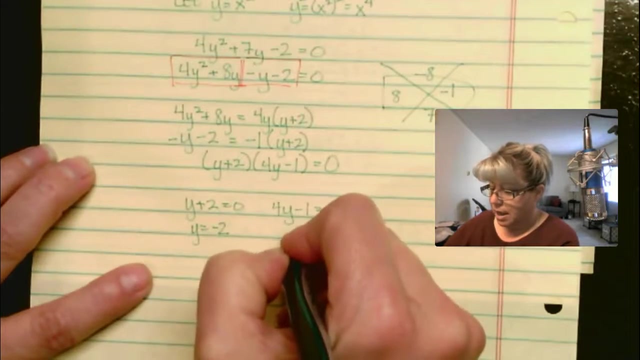 minus 1 equals 0. so let's use our 0 factor property to solve for y. Y plus 2 equals 0, 4y minus 1 equals 0, y equals negative 2 and for y equals 1. therefore, a y equals 1. fourth, but in the very beginning we start. in the coming sequence. we start with the second multiple on the bottom of the square, then we start to get hyperbolic term, we start to get the modPLUS A and by doing this we fix it up. So this plus 2 equals negative, 2 for y plus 1 equals 0. Y отличath 1 equals 1 less or minus 5. for y отличath minus 1 zero. 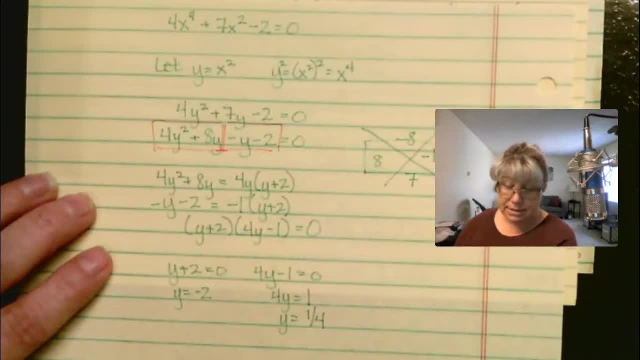 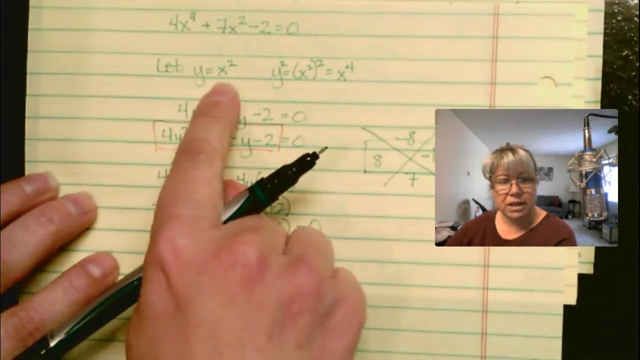 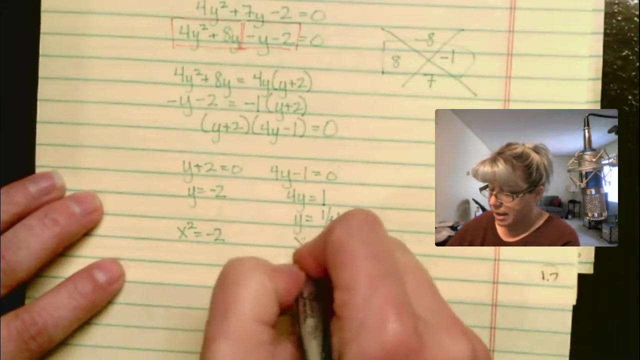 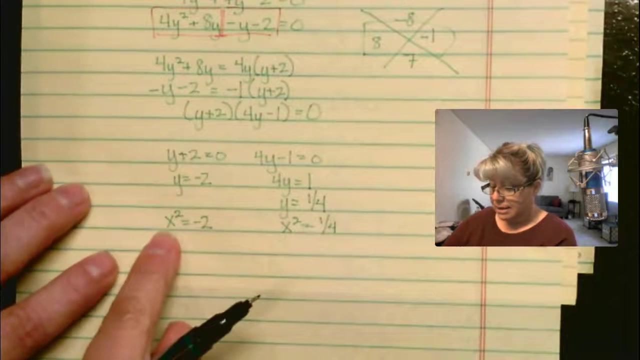 all the positive. this was a four week f. English started off with X's, not Y's, so let's go ahead and substitute back in. wherever we see a Y, we'll put an x squared. that means x squared equals negative 2 and x squared equals 1- 4. okay, x squared. I'm going to take the square. 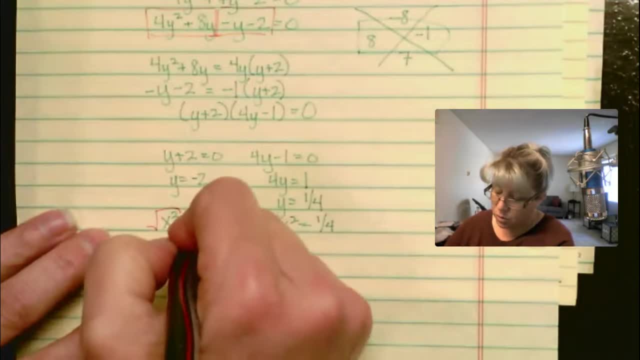 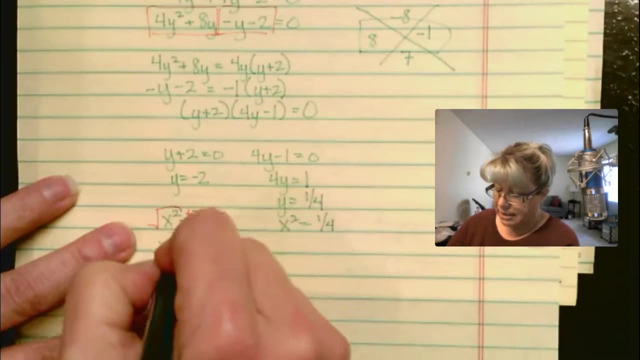 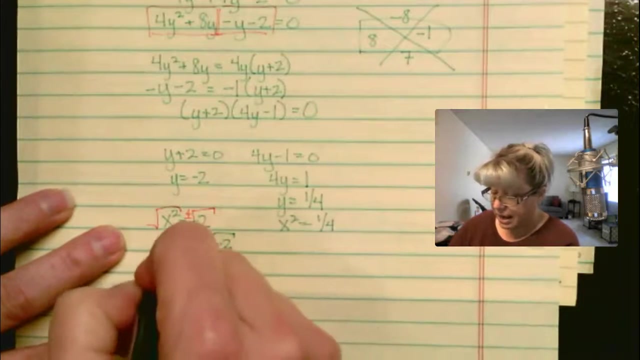 root of both sides, the square root of x squared, the square root of negative 2 plus or minus. let's not forget that on the right hand side, x equals plus or minus the square root of negative 2, but I can rewrite that as: x equals plus or. 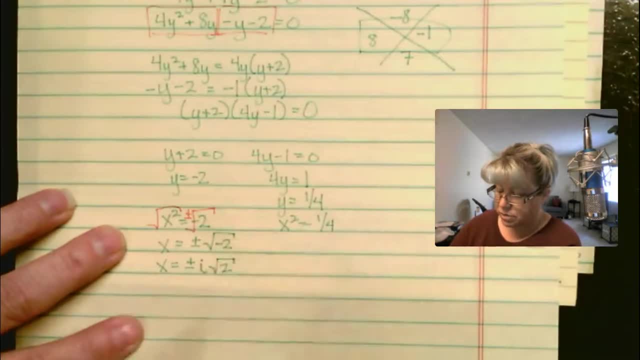 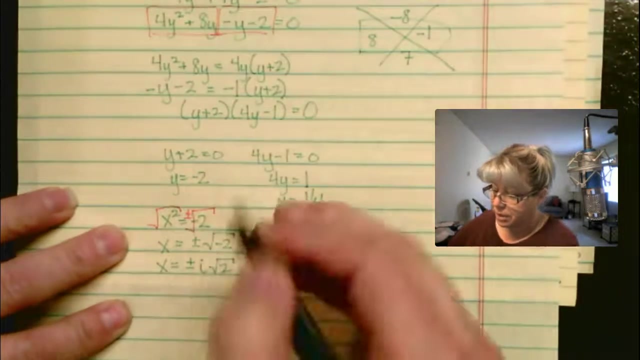 minus I square roots of 2. okay, all right, now let's do the same thing for our other possible solution. take the square root of both sides. right hand side is plus or minus. x equals plus or minus the square root of 1- 4, but the square 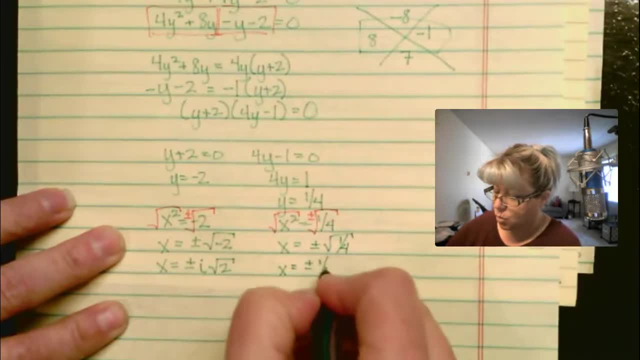 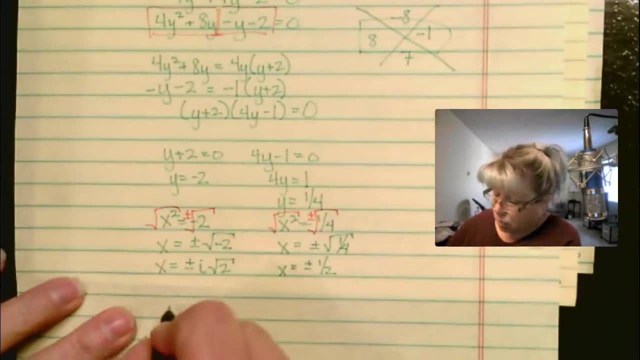 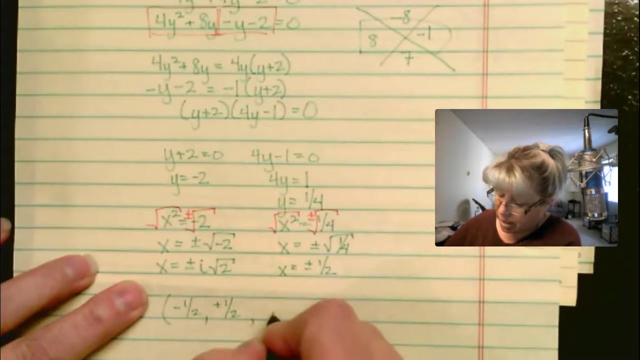 root of 1. 4 is plus or minus 1 half, so we actually have four possible solutions. X can equal negative 1 half, positive 1 half. could it be negative- I square roots of 2. or positive: I square roots of 2? you don't need the positive symbol there, I'm. 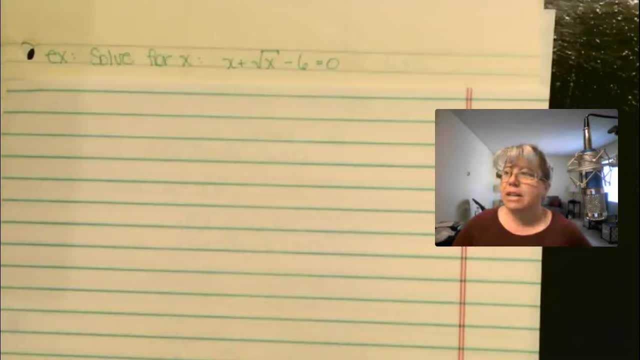 just using it for emphasis. another type of problem that we can use this substitution method is when we have square roots in there. now we have other means of figuring out square roots, but I'm going to use first substitution and then I'm going to use that other method and show you both ways. right, I'm going. 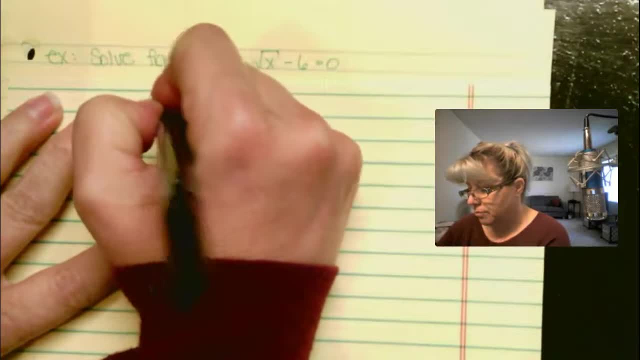 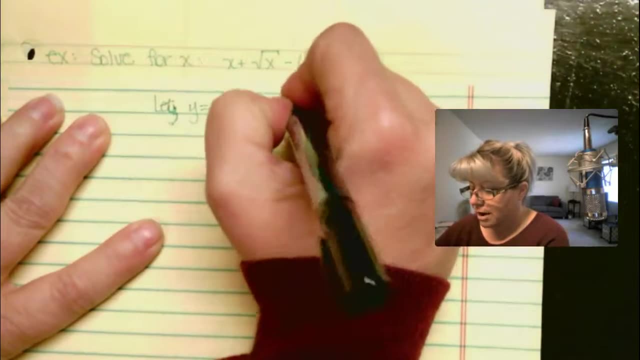 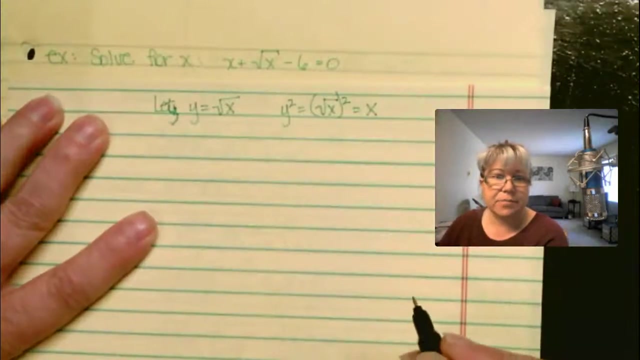 to let you know what I'm going to do is: I'm going to take the square root of x and I'm going to write down the square root of x, and I'm going to write down the square root of x and I'm going to write down the square root of x and I'm going 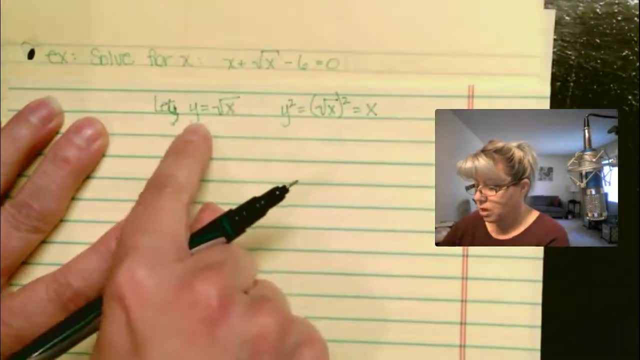 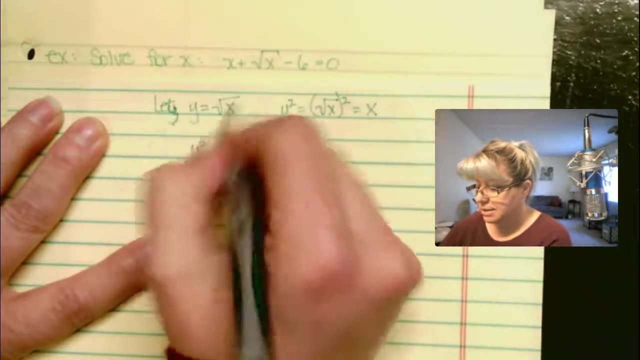 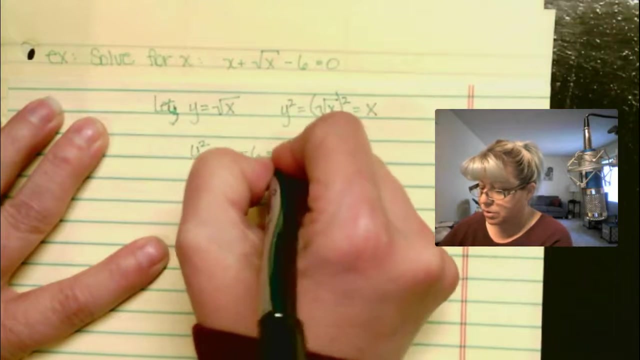 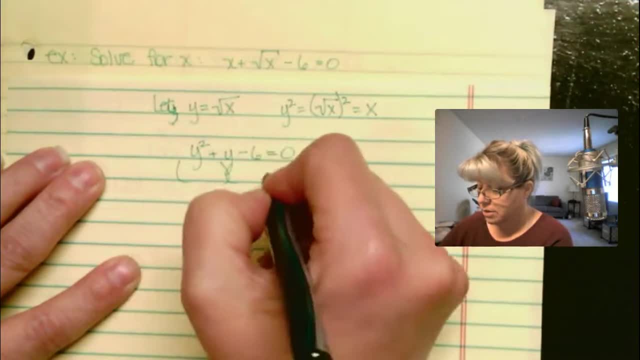 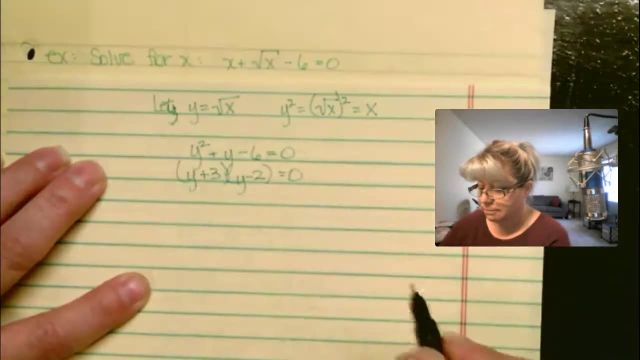 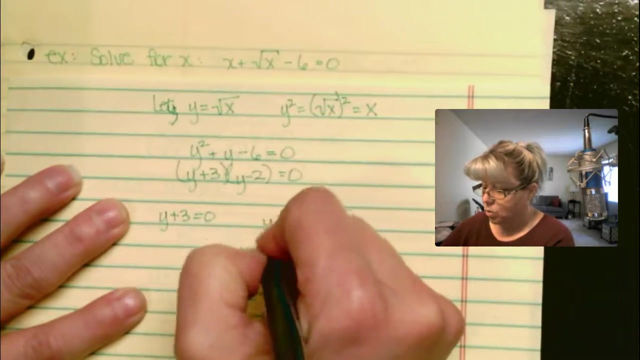 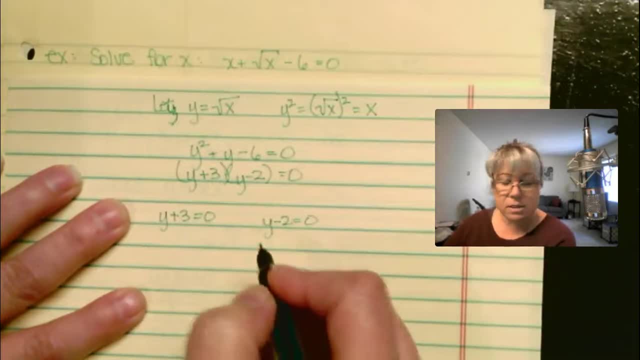 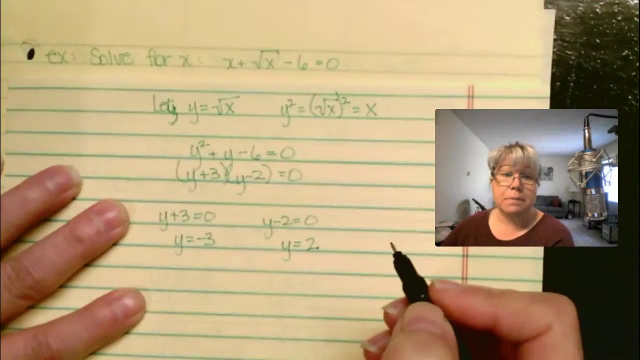 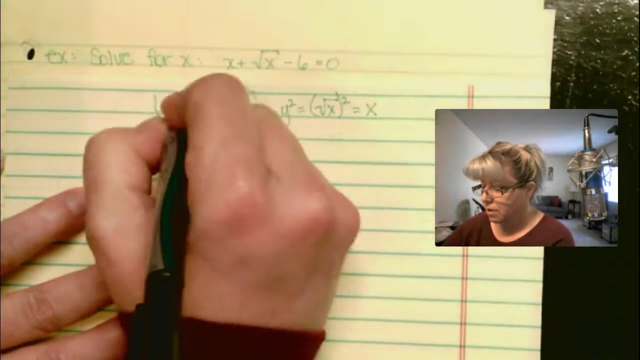 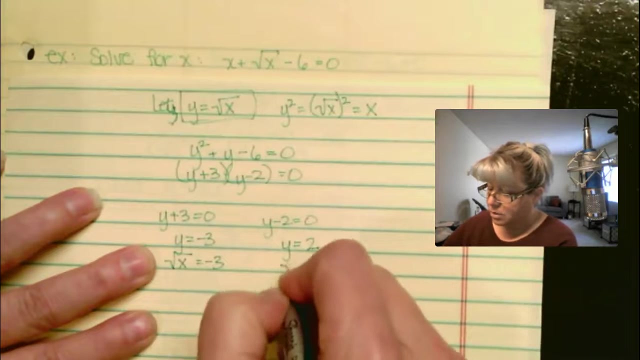 is 2 equals 0.. Therefore, our possible solutions: y equals negative 3 and y equals 2.. But again, my problem started with x's. it didn't start with y's. So wherever I see y, I'm going to substitute back in the square root of x. The square root of x equals negative 3 and the square root of x equals. 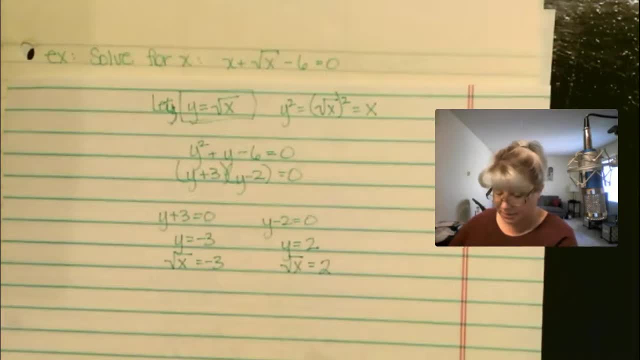 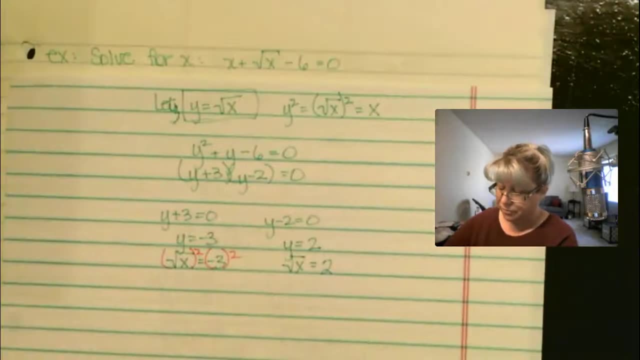 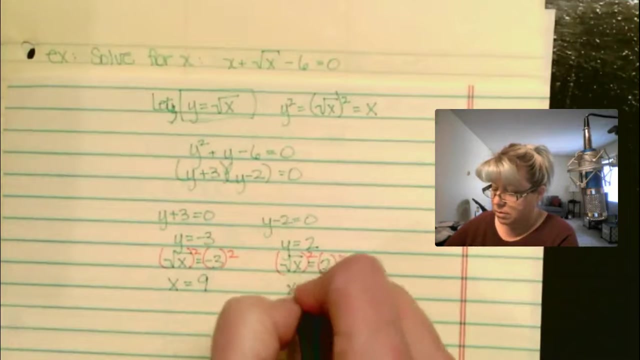 2 and I'm going to solve for x. That means to get rid of the square root. I need to square both sides. x could equal 9 because square negative 3 squared is 9 or x could equal 4, but because I raised x to, 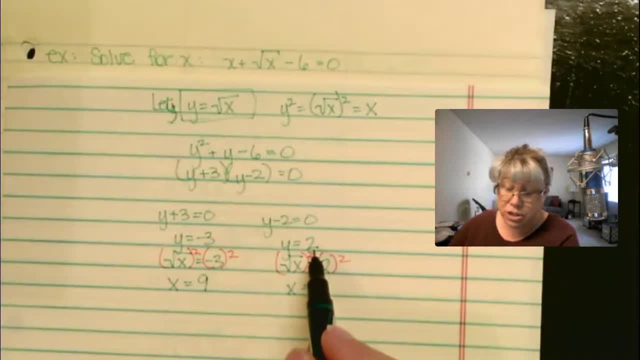 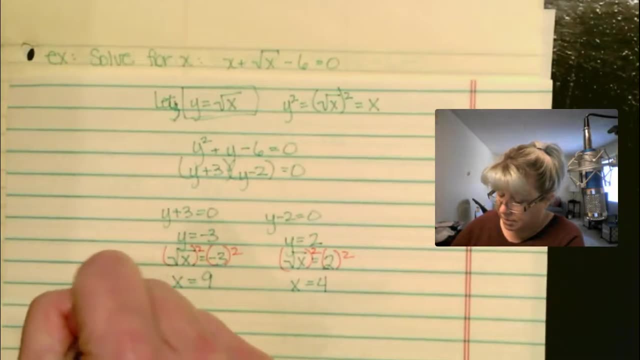 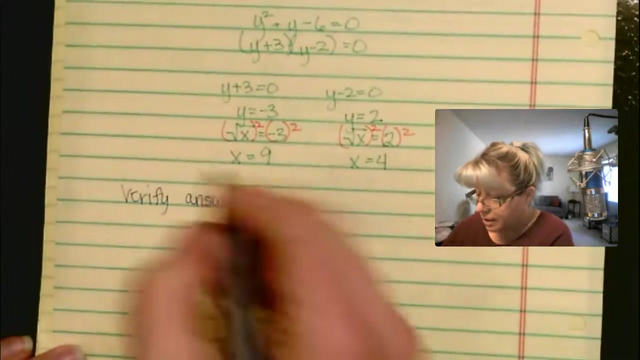 a square root, I need to square both sides. So I'm going to solve for x and I'm going to solve for squared power. I do have to verify that my solutions work for the original problem. I'm just going to verify my answers for X plus the square root of X. 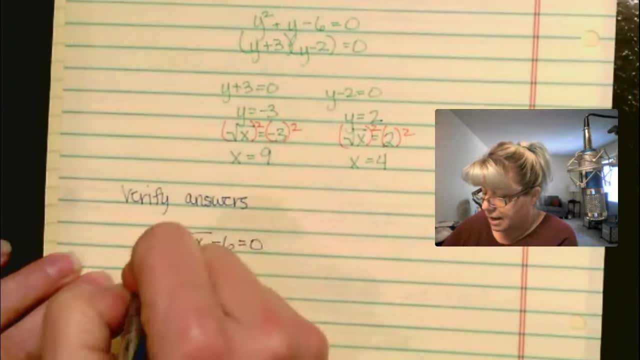 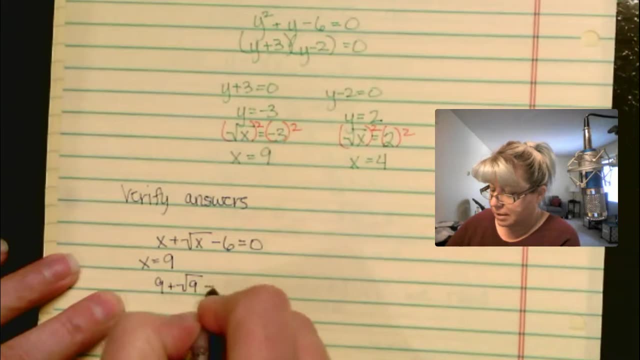 minus 6 equals 0. let X equals 9, therefore 9 plus the square root of 9 minus 6 does that equal 0. 9 plus 3 minus 6. 9 plus 3 is 12 minus 6 and 12 minus 6. 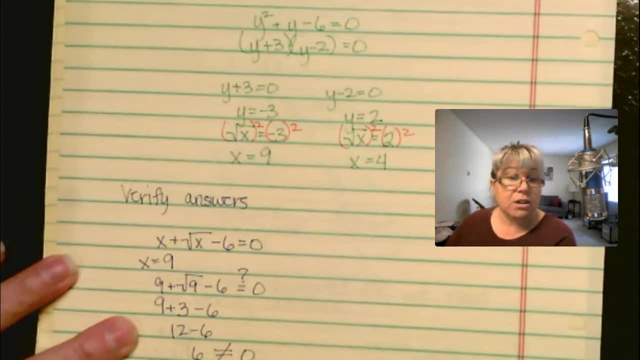 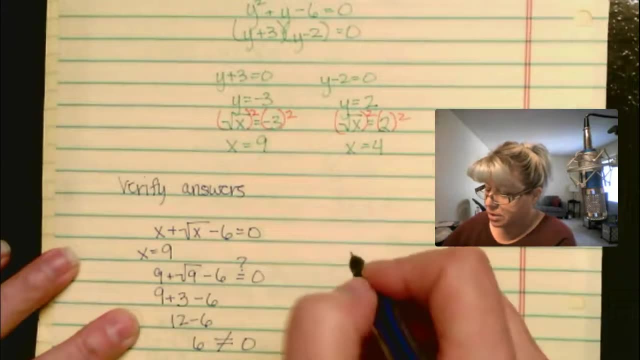 is 6. 6 does not equal 0, so X equals 9 is 0.. not one of our solutions. so let's try: x equals 4, 4 plus the square root of 4 minus 6 does that equal 0, 4. 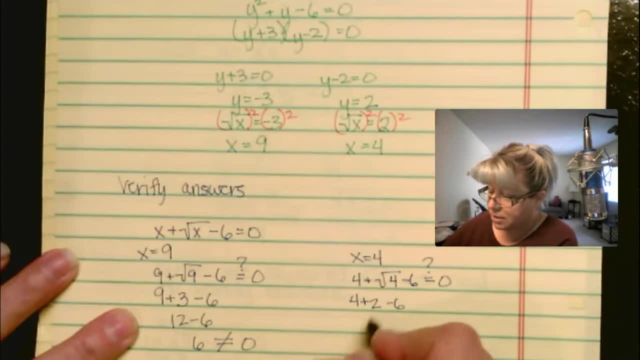 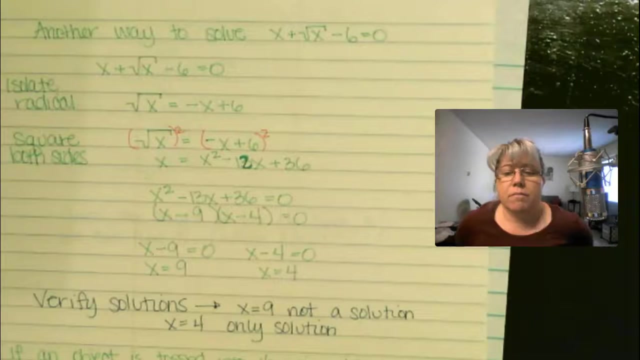 plus square root, 4 is 2 minus 6, 4 plus 2 is 6 minus 6 and 6 minus 6 is 0. so 4: x equals 4 is our only solution equation and 3 is our solution solution. solution x equals 9 was an erroneous solution. The other way to solve this problem would be to 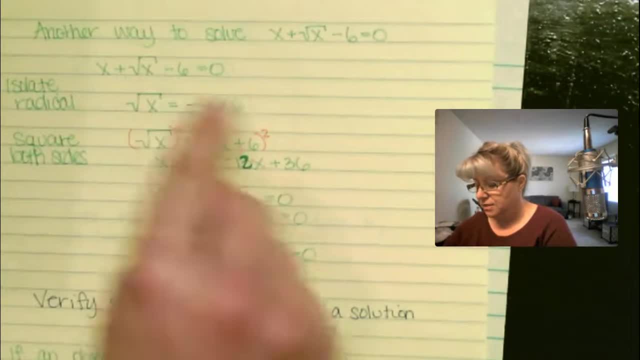 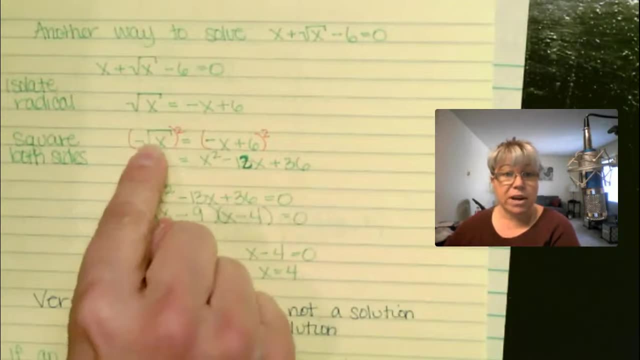 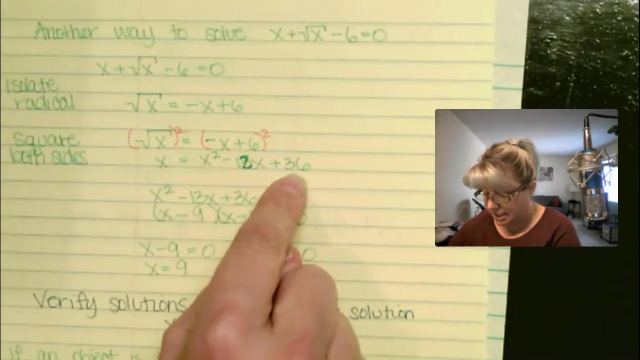 isolate the radical. So let's move the x and the negative 6 over to the other side. So I get square root of x equals negative x plus 6.. Now I'm going to square both sides, giving us x equals x squared minus 12x plus 36.. Let's move everything to one side: x squared minus 13x plus 36 equals. 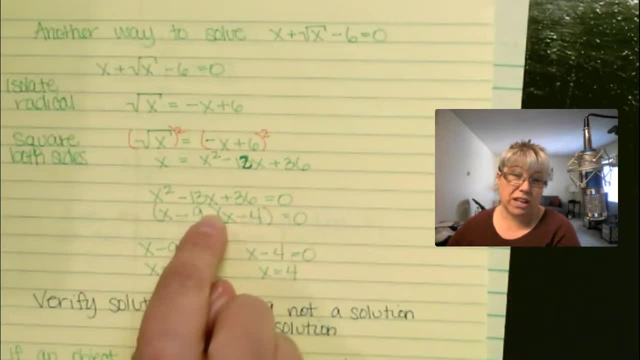 0.. And now we can factor our quadratic equation here: x minus 9, x minus 4 equals 0.. Let's solve each factor to 0 using the zero factor property. x minus 9 equals 0,, therefore x equals 9.. 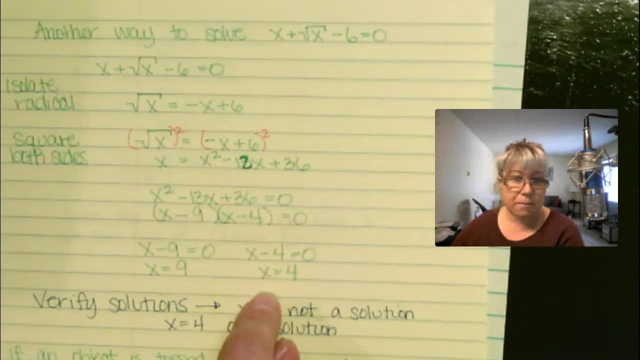 x minus 4 equals 0,, therefore x equals 4.. Again, because I did this squaring both sides method, I do have to verify both solutions And the process is exactly the same as before. So x equals 9 was not a solution and x equals 4 was our only solution. 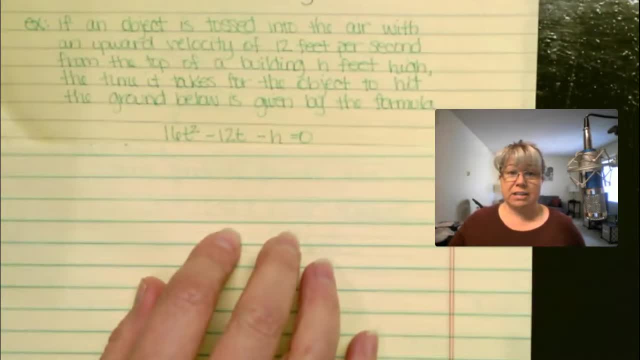 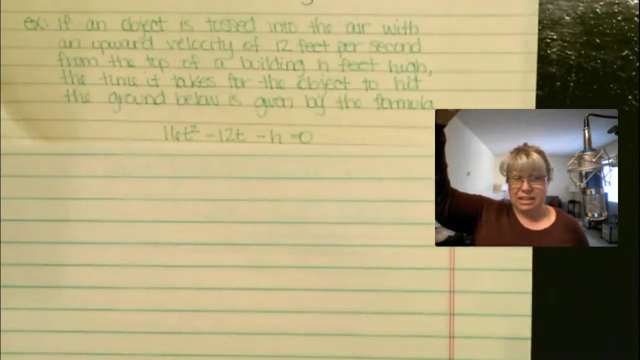 All right, let's say you toss an object into the air with an upward velocity of some speed. We'll say that it's 12 feet per second. We're throwing it from the top of a building that is 8 feet high. We want to know what time it takes for that object to hit the ground. 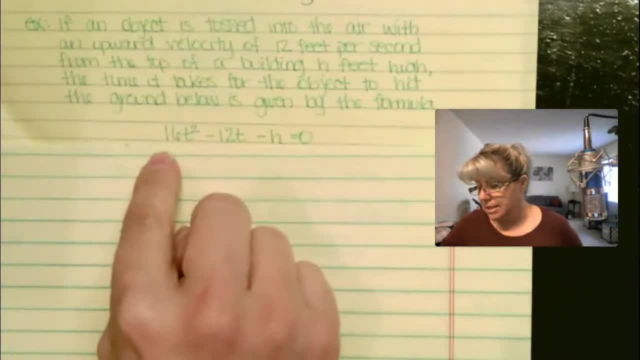 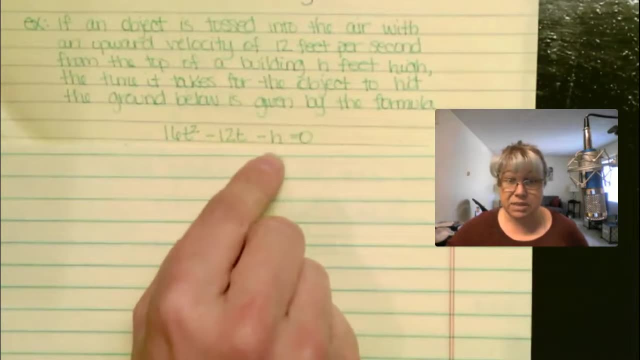 So here's our formula: We're given 16t squared minus 12t, minus h, being the height of the building equals 0. And I want to know, I want to solve this equation, to get the height of the building. So I'm going to use an x equation. Well, what is an x equation? 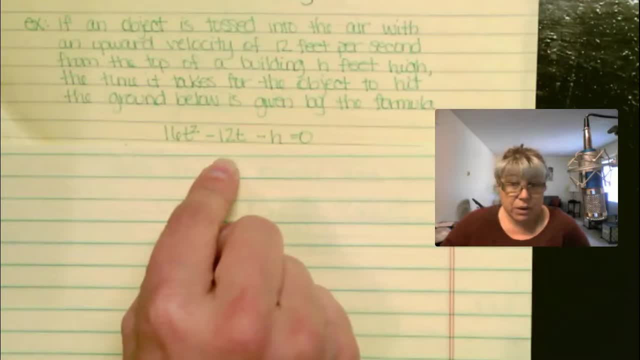 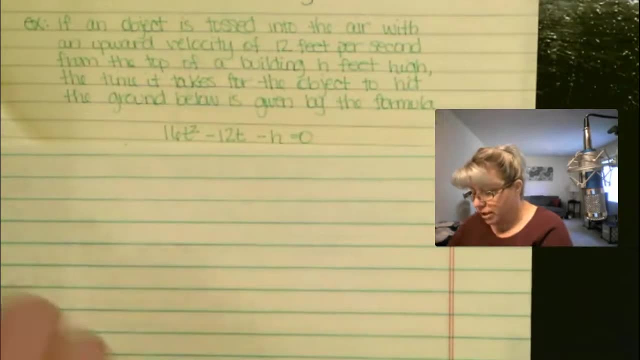 An x equation is C, the volume, and. but we still need to solve to get to the solution. So I'm going to use an x equation for t. Well, this is just a quadratic equation. That's it, Quadratic equation. So I'm going to go ahead and use the quadratic formula to solve for h. 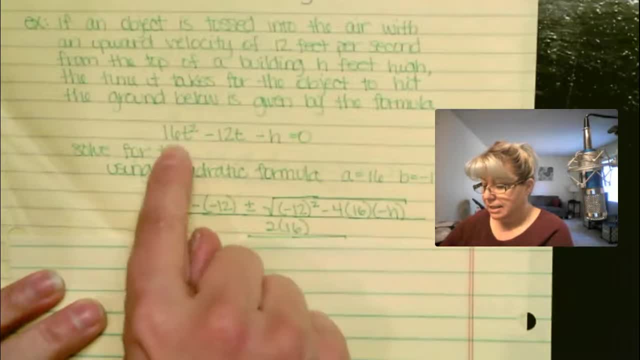 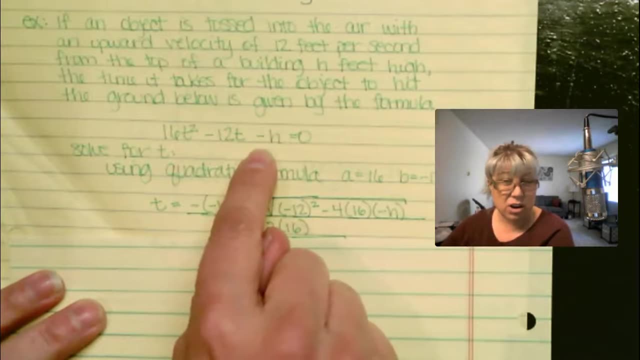 Now a quadratic formula. we usually use x equals, But I'm going to use t equals because I'm solving for t here h. I'm not going to worry that there's an h in there, I'm just going to keep solving for t, So plugging all of the a, b, c. 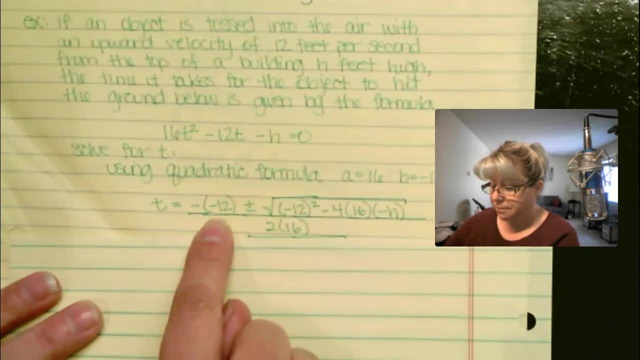 into our quadratic equation the values for a, b, c minus, pardon me, negative, negative 12 plus or minus the square root of negative 12 squared minus 4 times 16 times negative h, all over 2 times 16.. 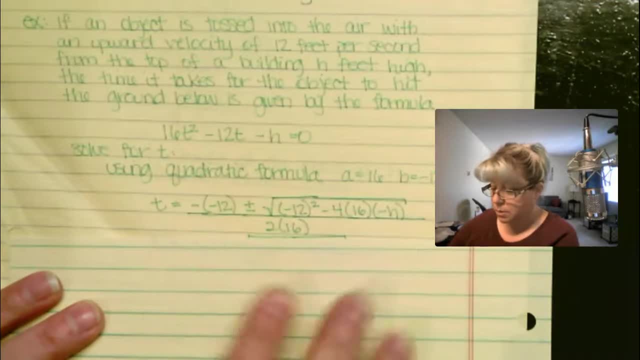 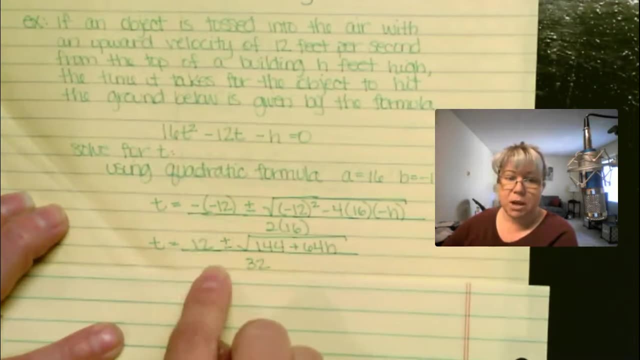 I'm going to simplify this as much as possible: Negative 12, negative, negative. negative 12 is positive 12.. Negative 12 squared is 144 and negative 4 times 16 times h is going to be a positive: 64: h 2 times 16. 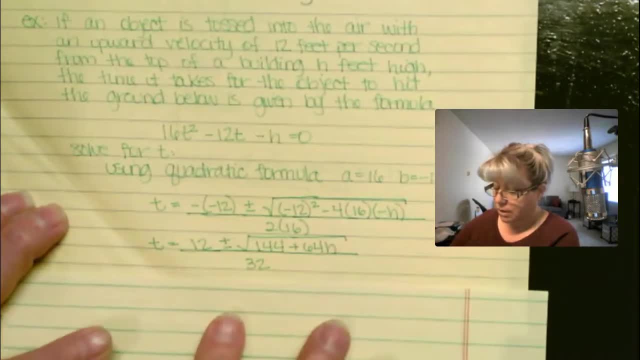 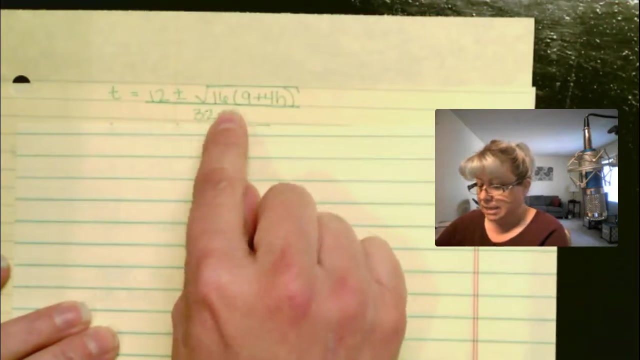 is 32.. Now I can factor the radicand here. If I factor, I'm going to end up getting 16 times 9 plus 4 h 16 is a perfect square. so I can pull out the perfect square here, which is 4 squared. 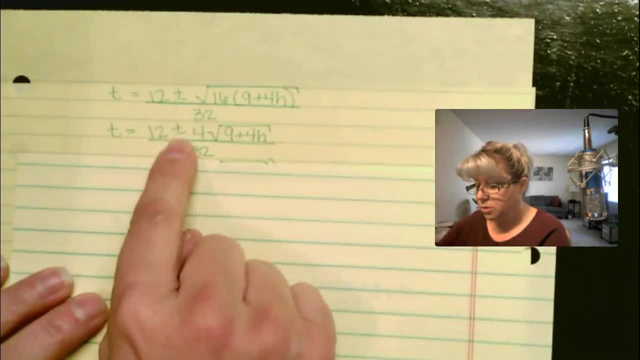 That will give me: t equals 12 plus or minus 4, square root of negative 12.. So I'm going to take the square root of 9 plus 4 h, all over 32.. But I can factor the numerator. I can pull out a 4 out of a 12 and a 4 out of a 4. 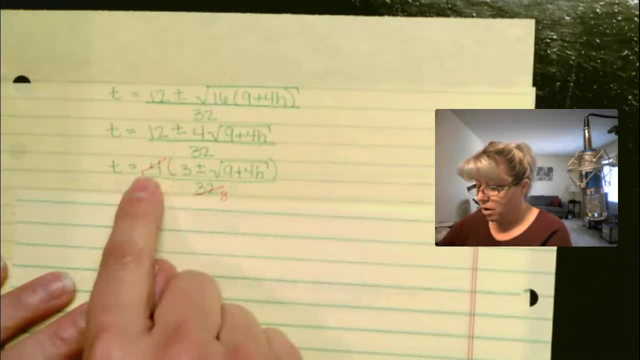 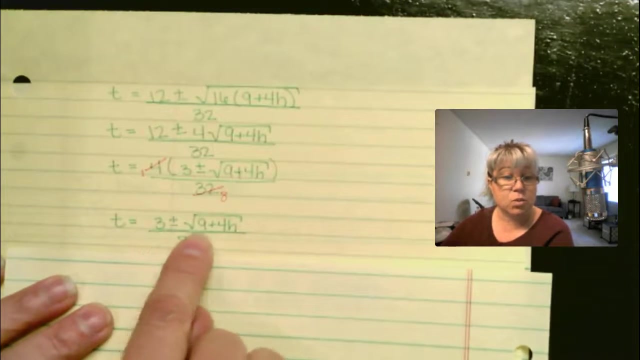 and say 4 times 3 plus or minus the square root of 9 plus 4 h, all over 32.. And the 4 and the 32 can reduce. Giving me t equals 3 plus or minus the square root of 9 plus 4 h, all over 32.. 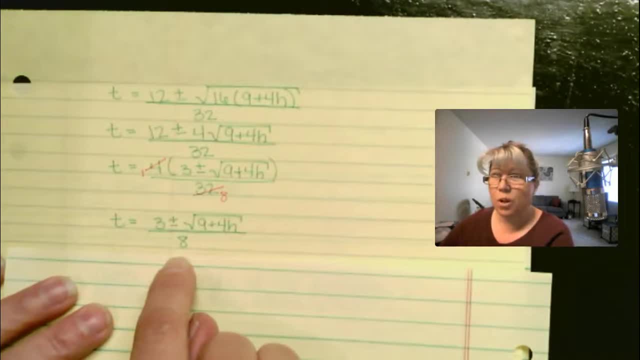 So I get 4 h all over 8.. Now, how does that help me? I didn't necessarily solve for time, but if I am given the height of the building, I just plug that in and I'll know exactly what time it will. 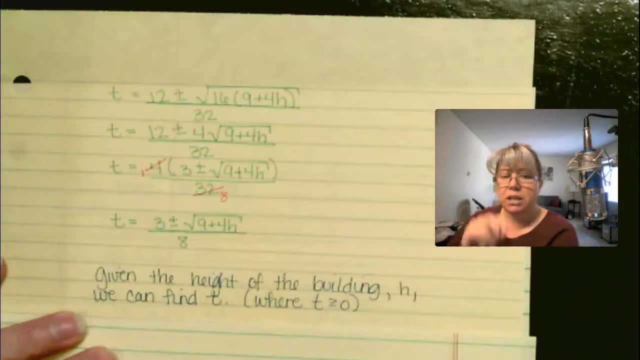 take for that object to hit the ground. Generally speaking, you will have two values of t. Remember, with our determinant, we will either have two complex answers, two irrational answers, two rational answers or one rational answer Generally, we'll have two rational. 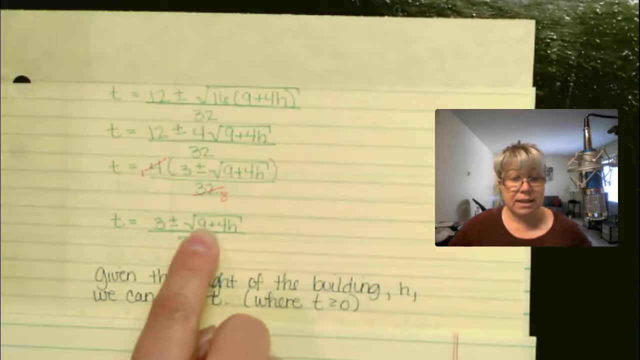 answers, because this will be either two rational answers or two irrational answers, because the determinant here will be positive. The building height is always positive, So this value will always be positive, Because one might be. if we solve for t, we have 3 plus this positive. 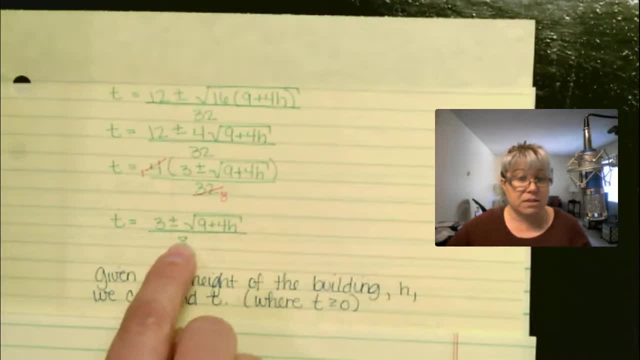 this positive number equals 8.. 3 minus this positive number minus all over 8.. We're just looking for the value of t, which is positive. The t that is the negative we don't care about, because time isn't negative, time is positive. 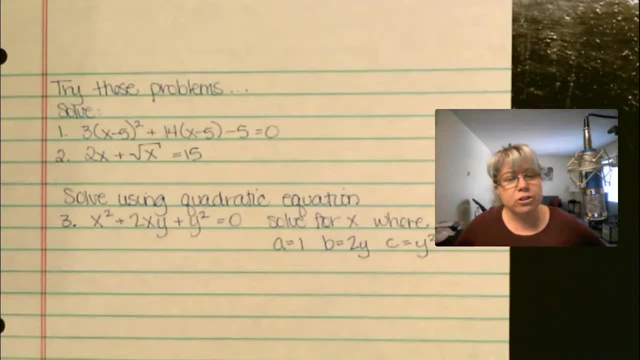 Alright, so that's it for this lecture. Why don't you go ahead and try these problems yourself? Go ahead and solve 3 times x minus 5 squared 14. x minus 5 minus 5 equals 0.. Try using the substitution method here. 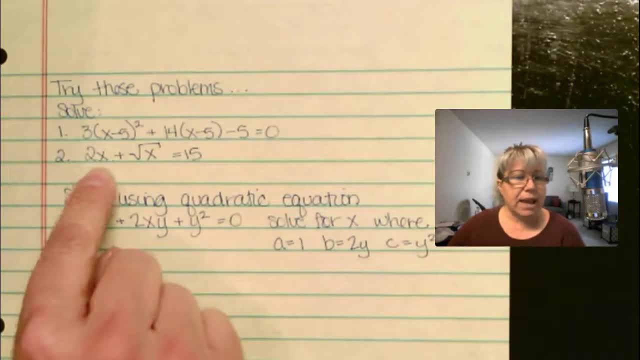 Likewise with number 2.. 2x plus the square root of 2 equals 15.. First, set it in standard form and then go ahead and use substitution. I think it will work for you. And then, solving the third problem, go ahead and solve using the quadratic.